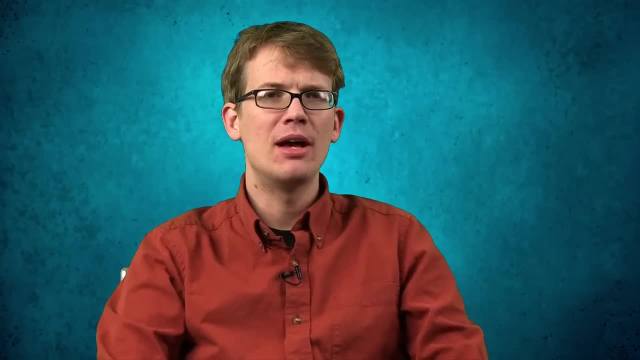 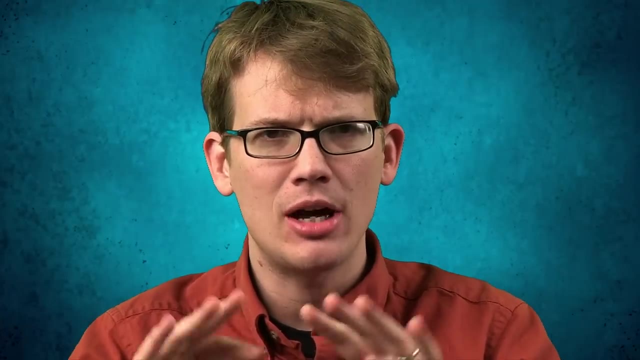 Ah, that would suck to have to wear that all the time. So you never know when the next mass extinction is going to happen. I mean, there have been five of them in the last 450 million years alone, And it's not like a mass extinction is some kind of blurry, ill-defined term. It's when at least 50% of the species on the planet go extinct. One of them, which has been aptly dubbed the Great Dying, wiped out more than 95% of the species on the planet. It's enough to make you walk around with a gas mask. It's possible that the gas mask is excessive. It's also possible that it's useless. I mean, if we get hit by a big meteor, probably not going to help that much. Mass extinction events happen pretty fast in a geological way, But the actual like dying occurs on our scale quite slowly, tens of thousands of years. And of course the most important thing to look at here is what these five giant mass extinction events had in common so that we can see them coming. 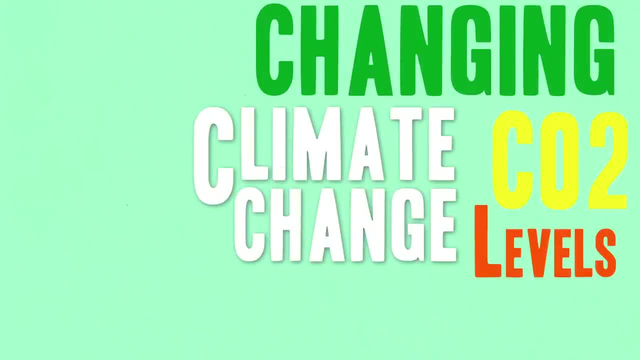 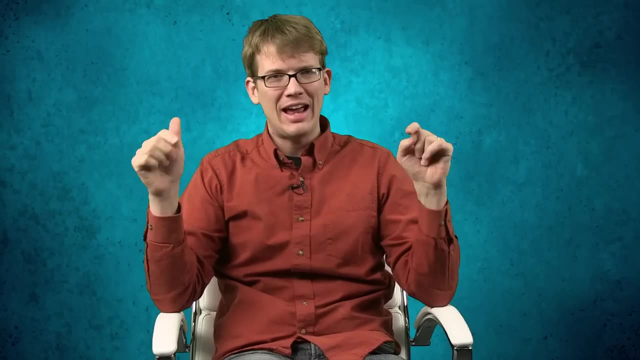 Climate change, usually caused by changing CO2 levels and relatively rapid global temperature changes. Yeah, so you see where I'm going with this. I don't mean to alarm anyone here, but the idea that the Earth is currently, as I sit here, going through a sixth mass extinction event is actually not that crazy. 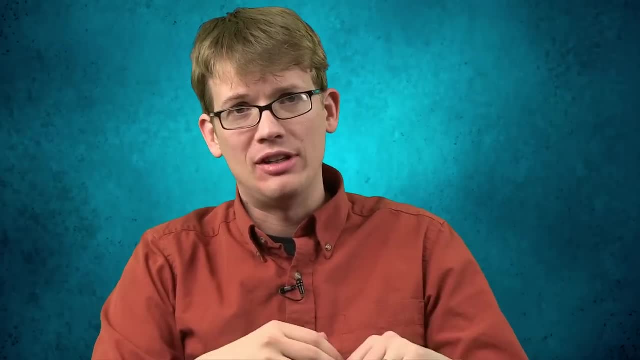 Yeah, so you see where I'm going with this. I don't mean to alarm anyone here, but the idea that the Earth is currently, as I sit here, going through a sixth mass extinction event is actually not that crazy. Scientifically, it actually might make really good sense. 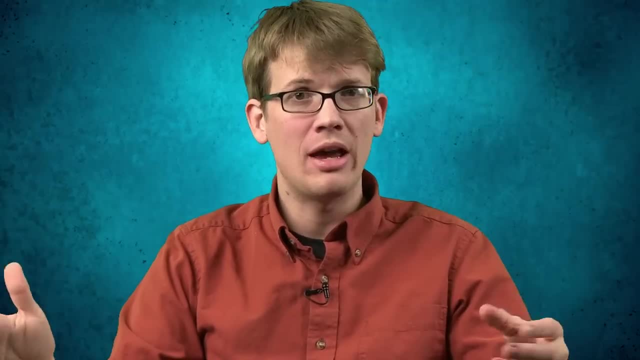 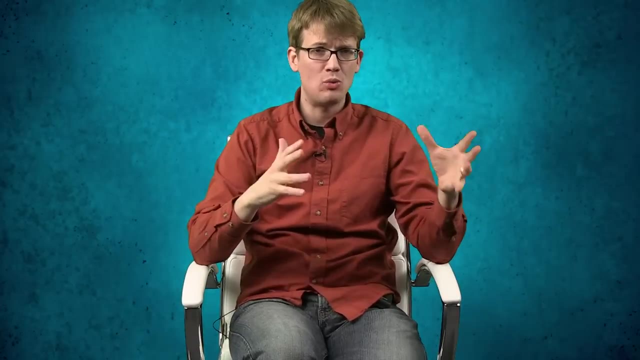 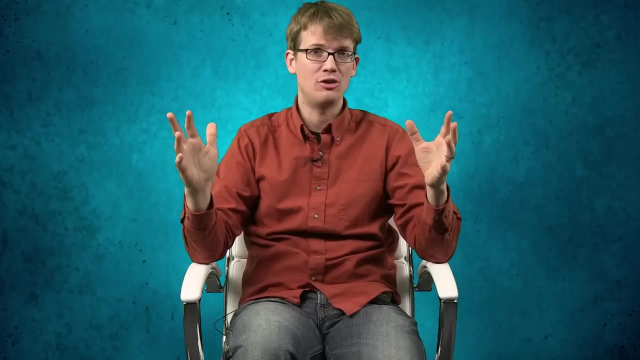 Before we even look at climate change, we already know that humans have been a strange and mysterious and new force for mass extinction. Current extinction rates are somewhere between 100 and 1,000 times what they would be naturally due to humanity's very enterprising nature. 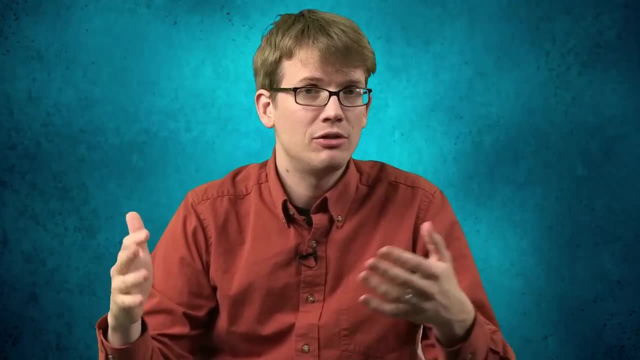 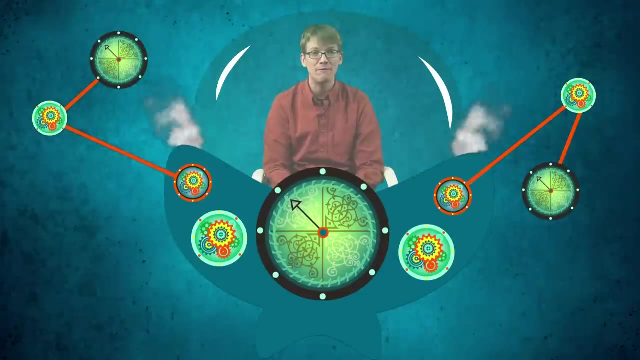 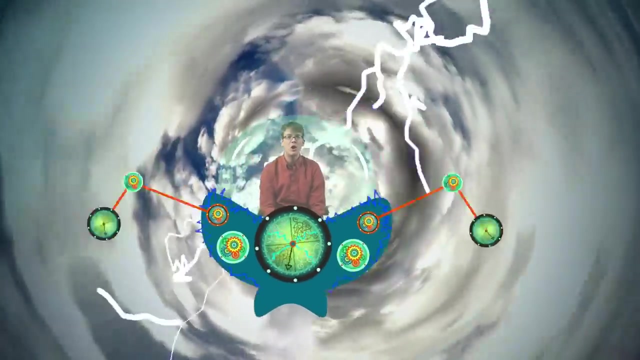 And that rate is similar to, or even greater than the rates of some mass extinction events of the past. So let's forget about all that depressing stuff for a moment and hop into The SciShow Time Machine. Our first stop 450 million years in the past, and we're gonna get a little bit wet, because pretty much all life on Earth at that time was in the oceans. 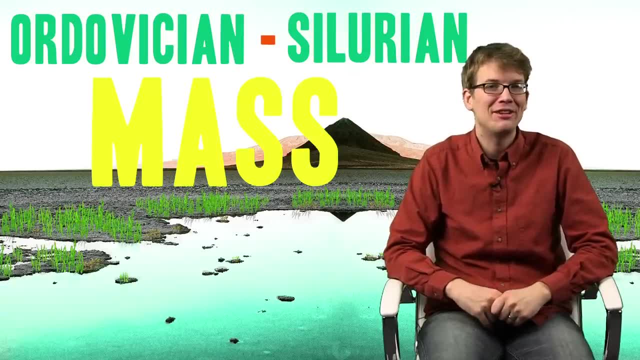 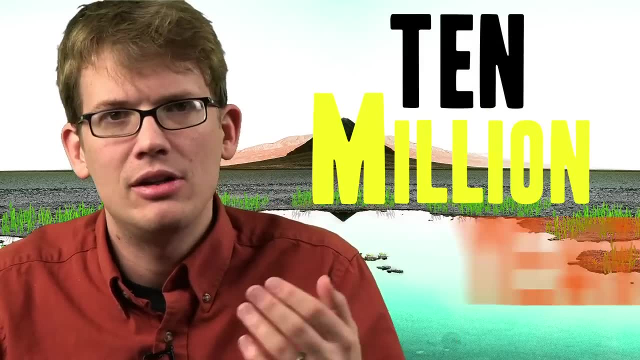 Welcome everyone to the Ordovician-Seluvian mass extinction event. Now you're not going to see any giant comets or meteors falling from the sky, But sometime in the next 10 million years or so we're gonna see two really dramatic die-offs. 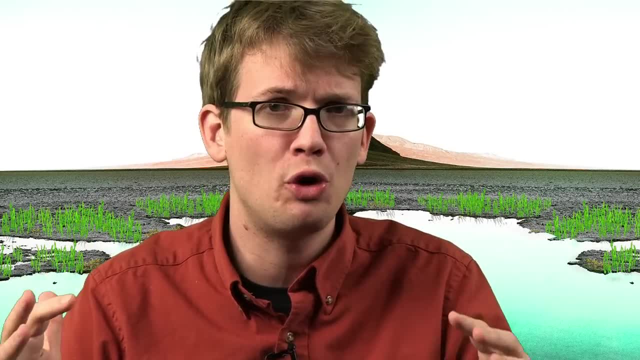 Both of them involving the influx of gigantic glaciers and dramatic worldwide earthquakes. Both of them involving the influx of gigantic glaciers and dramatic worldwide earthquakes. Both of them involving the influx of gigantic glaciers and dramatic worldwide earthquakes. Both of them involving the influx of gigantic worldwide earthquakes. 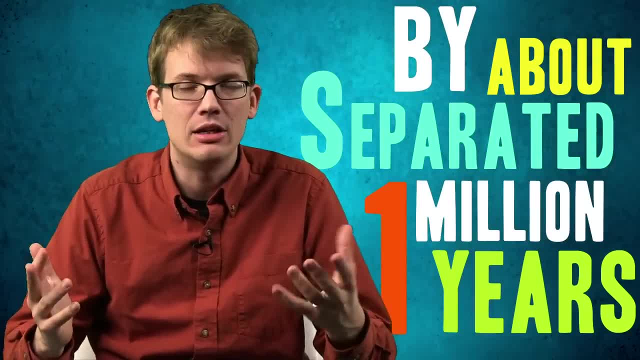 Both of them involving the influx of gigantic worldwide earthquakes. The 거야이고 kurWorld pela Shrun mbklalustruj I trickisiçłangingereumärča İf бы Dåp cease هناκιем. 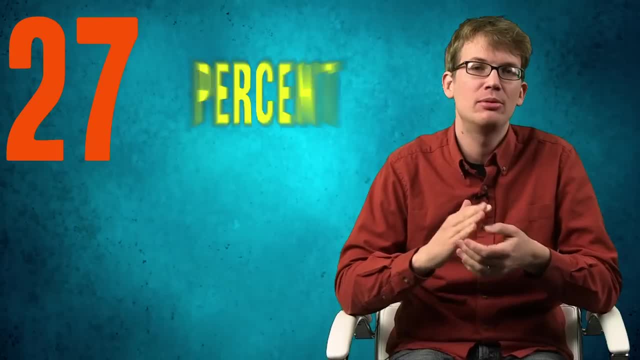 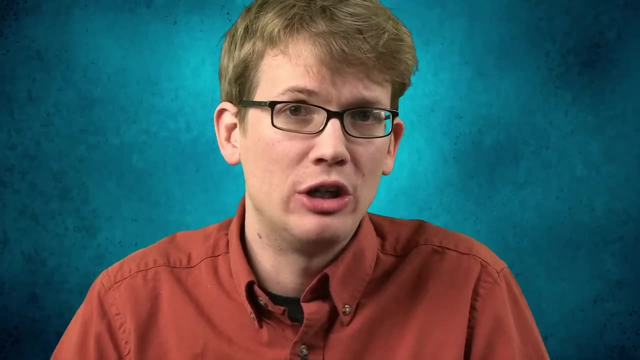 And it's a geologic time, remember people. And by the end of the second one, 27 percent of All Marine families and 60 percent of All Marine genera were extinct, And I can tell from your blank stares that we're going to require a little bit of a refresher. 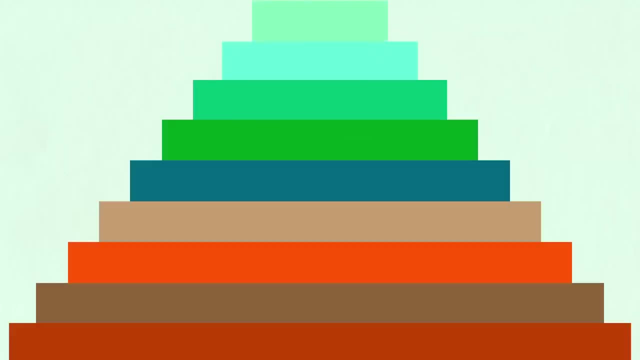 on the biological classification system which, of course, classifies our life based on common descent, and which we will be talking a lot about as we get more into extinction events, Starting with the most specific and then getting to the most general. we have 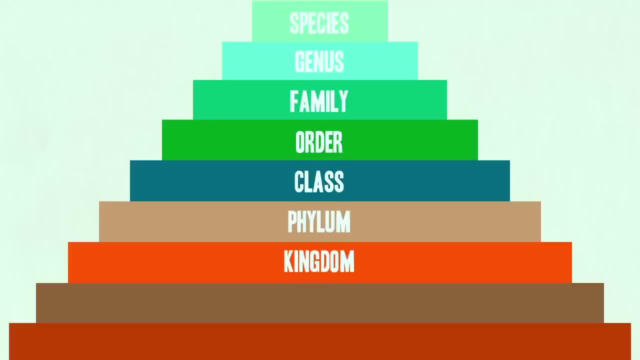 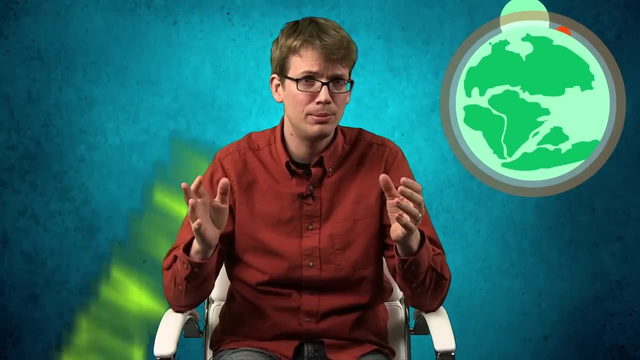 Species, genus, family, order, class, phylum, kingdom domain and good old life. Back to the Ordovician event. what scientists think happened here was that Gondwana, one of the two supercontinents at the time, moved into the polar region. This set off a huge drop in temperature, also a huge increase in glacial formation, which dropped sea levels. Marine invertebrates were the hardest hit. Two-thirds of all the brachiopod and bryozoan families disappeared. It was also a tough time to be a bivalve or a trilobite. 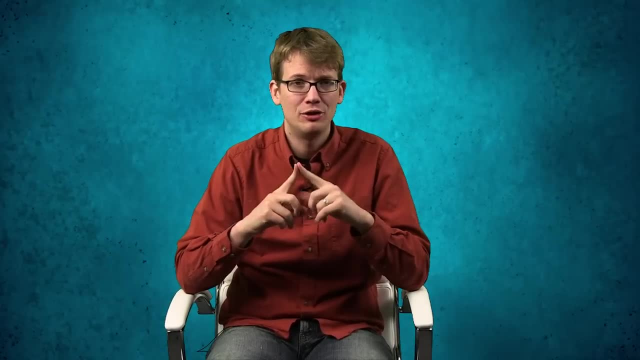 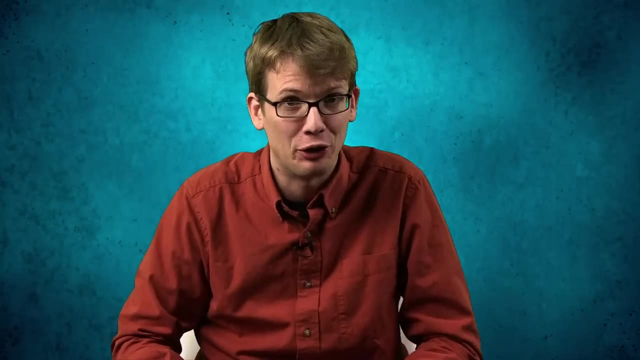 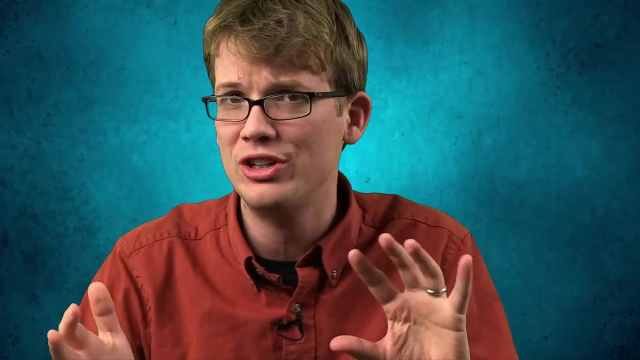 And just because I find this fascinating, there's also another theory about what may have happened to cause the Ordovician event: A gamma-ray burst from a hypernova somewhere within 6,000 light-years of Earth. A supernova: that's when a star explodes. A hypernova is when a star that's like 100 to 300 times the size of the Sun explodes. Even like 10 seconds of a gamma-ray burst from a hypernova would completely destroy the ozone layer and dose everything on Earth with a nice healthy amount of UV radiation. When I say healthy, I mean unhealthy. All right, everybody back in the time machine. 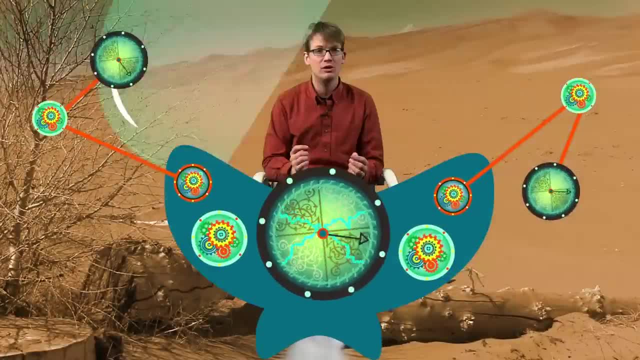 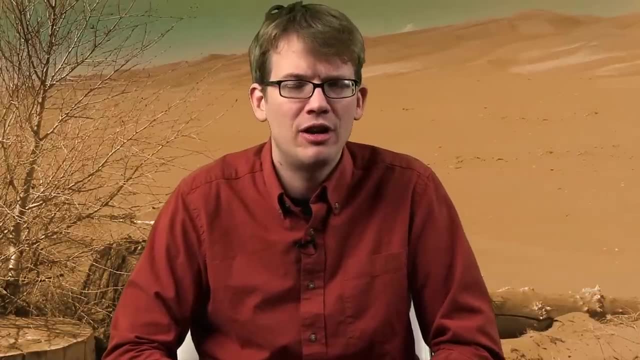 We're going ahead 100 million years to 360 million years ago, to the late Devonian extinctions. This is the beginning of a prolonged series of mass extinctions in which half of all genera and 70% of all species will go bye-bye. Marine life will once again be hit very hard, but so will the spiders and the scorpions and the proto-amphibians which are just taking their first steps out on the land. Narrowing down a time frame for this event has been difficult. Scientists can only say that over a period of 500,000 years, this event has been a very, very difficult event. Scientists can only say that over a period of 500,000 years, this event has been a very, very difficult event. 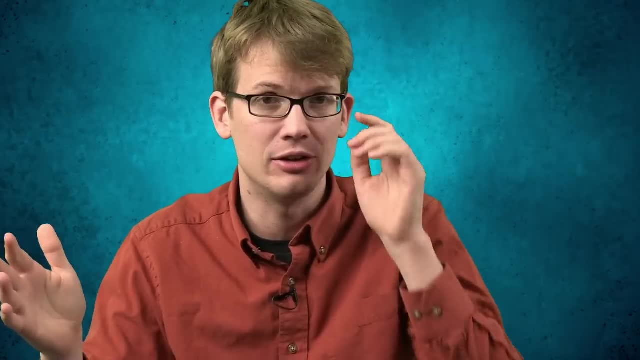 Scientists can only say that over a period of 500,000 years, this event has been a very, very difficult event. 500,000 to 25 million years- That's a big gap. there. I know There were a series of extinction pulses each lasting about 100,000 years. 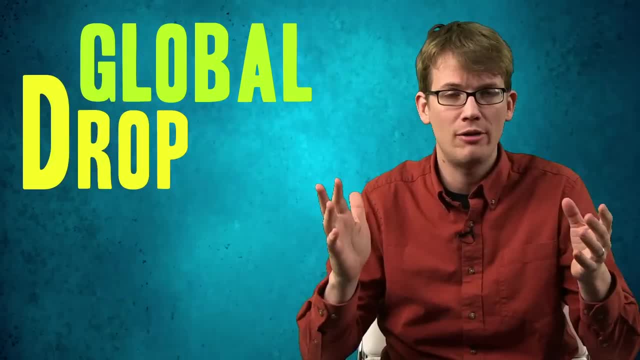 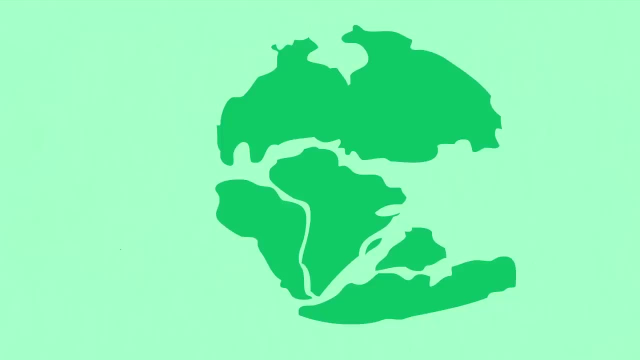 No gamma-ray bursts are suspected here. This is once again being caused by a global drop-off in temperatures. People aren't sure what caused it, Probably either an asteroid impact or a giant supervolcano. Each of those things would have released massive amounts of dust or ash into the atmosphere, drastically changing the climate. 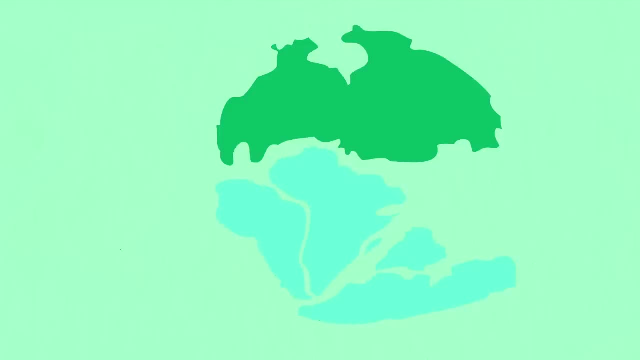 Glaciers probably once again inundated Gondwana. What we also know is that ocean levels fell and lost most of the ocean's surface, Most of their oxygen, in the process, in what's called ocean anoxia. Some believe that temperatures in the steaming seas of the Devonian fell from 93 to about 78 degrees. Coral reefs were hit so hard that it would be 100 million years before they recovered. But there's another interesting theory here, and that's that plants which were, for the first time, really taking hold on land were absorbing so much carbon dioxide from the atmosphere that they actually caused global cooling. 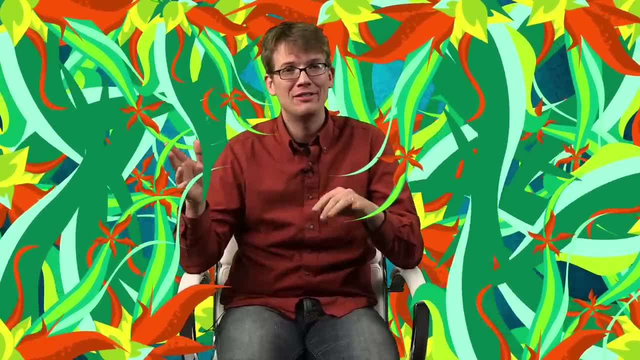 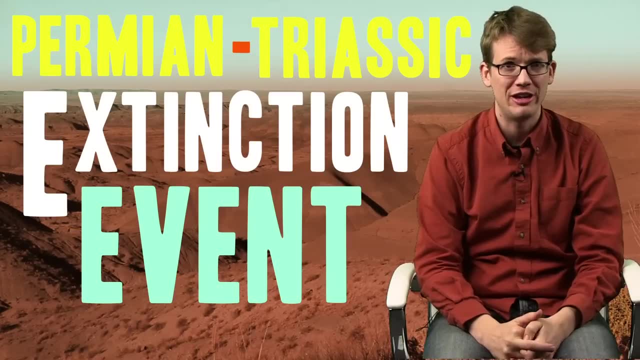 So, in fact, plants were responsible for that mass extinction event. How could you? And now we will travel to the big one, Also known as the Permian Triassic extinction event, Also known as The Great Dying. It is now about 250 million years ago. 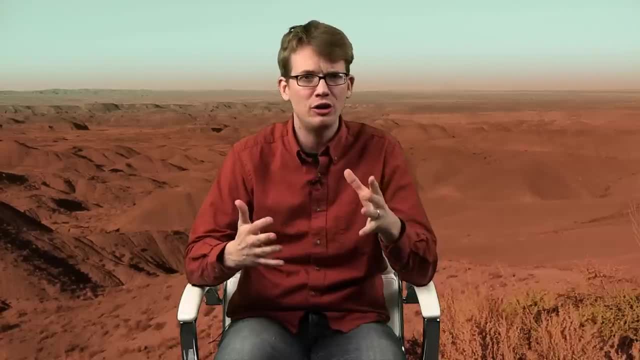 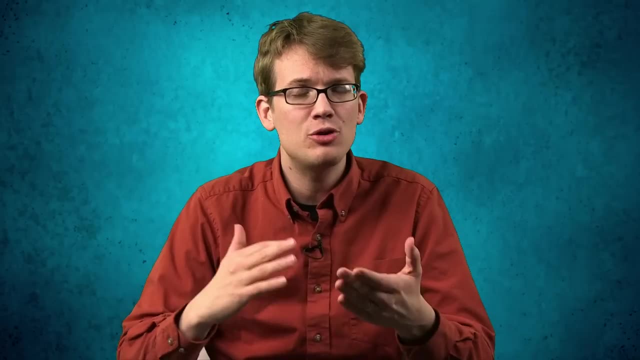 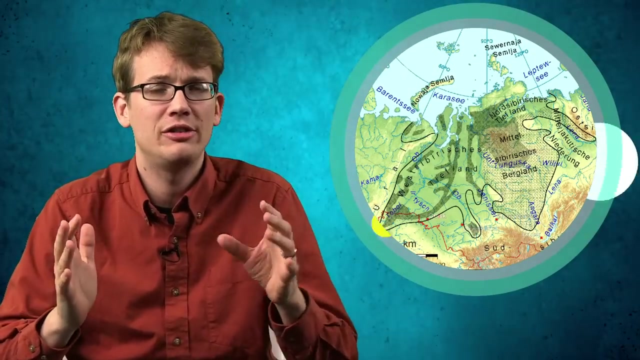 And a combination of catastrophic events is about to totally alter life on planet Earth. So destructive is this event that it remains the only known mass extinction of insects. This may have been triggered by a comet or asteroid impact, but what scientists feel fairly certain about is that a subsequent volcanic eruption in an area known as the Siberian Trapes 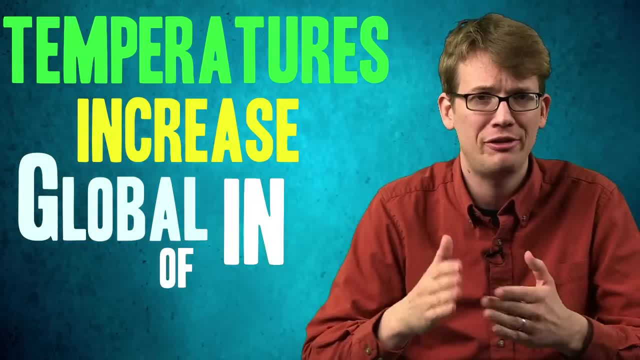 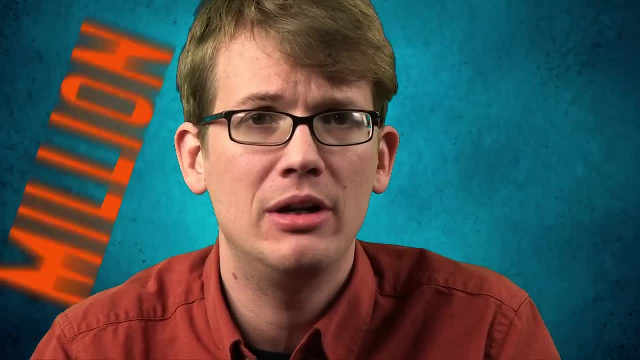 traps was responsible for an increase in global temperatures of 5 to 10 degrees. These volcanic eruptions covered an area roughly the size of Western Europe and they lasted for a million years, But then it got worse. The sudden release of gases from methane hydrate reservoirs below the seafloor possibly caused 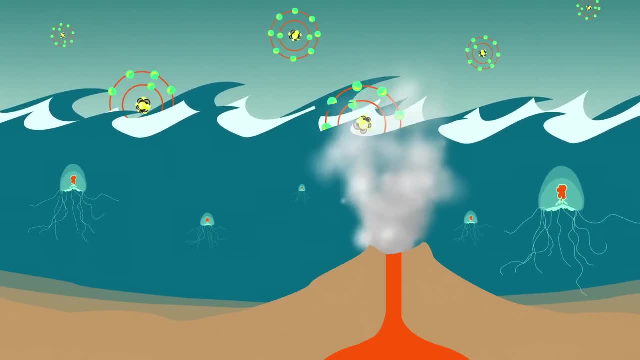 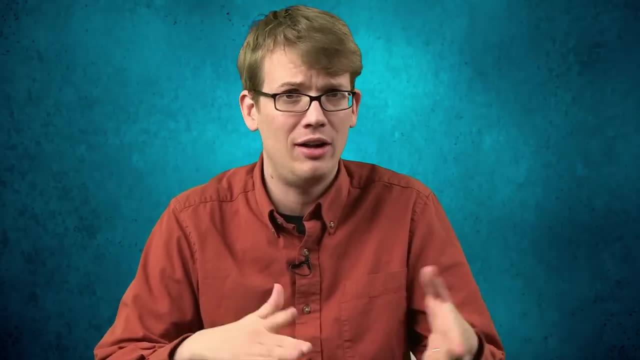 by underwater volcanic activity decimated the seas, leading to periods of too much oxygen, called hyperoxia, and too little oxygen, the return of anoxia, And marine life does not fare well in either of these conditions. These two events at least- possibly others- led to a shift in ocean currents and general 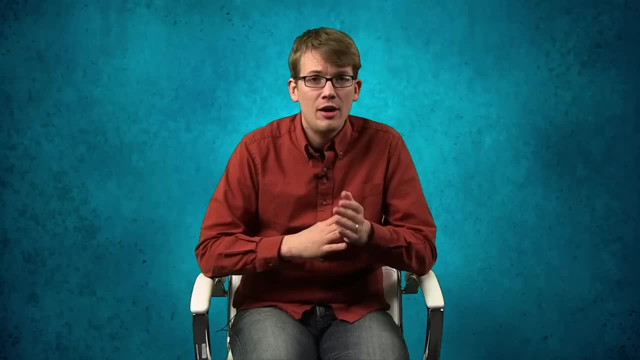 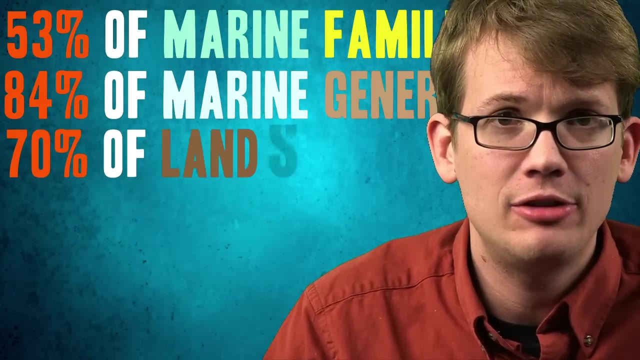 inhospitable environment for most of the Earth's species. When the die-off was finally finished, 53% of marine families, 84% of marine genera, 70% of land species and 95% of marine species were extinct. 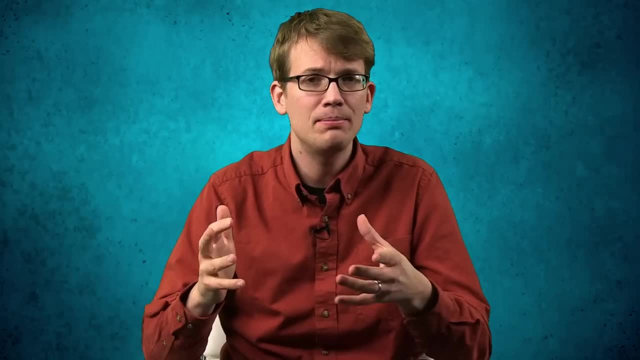 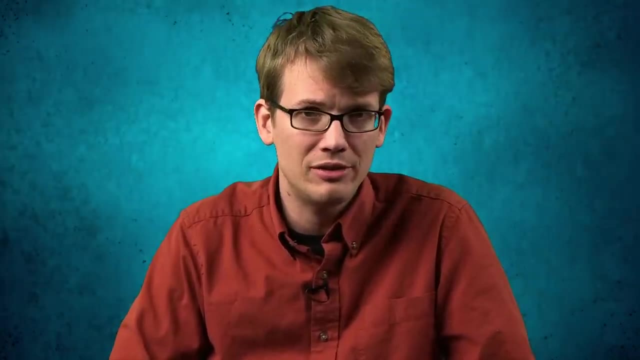 The Permian extinction had an enormous evolutionary effect, taking place just as mammal-like reptiles like pelicosaurs and therapsids were in their prime. It would be more than 30 million years before these vertebrates would be extinct And the Earth in general would recover. But it did recover until 200 million years ago, when the Triassic-Jurassic extinction killed off many early land animals. This includes the death of most of the therapsids, large amphibians and the archosaurs, paving the way for the age of the dinosaurs. Scientists probably know less about this mass extinction event than any other, but what is known is that 23% of families and 48% of genera went extinct, but what was left fairly untouched were plants and dinosaurs. These were dinosaurs which now had a lot less competition. This was roughly the time when the massive supercontinent known as Pangaea was breaking apart due to volcanic eruptions, And the massive release of carbon dioxide from those eruptions may have caused some pretty intense global warming Again. species don't fare well when temperatures increase quickly like this. And it wouldn't be an extinction event without scientists wondering about whether or not there was a massive impact of some kind. But so far nobody's found any likely crater candidates. But you know where there is evidence of an impact crater: Right off the coast. 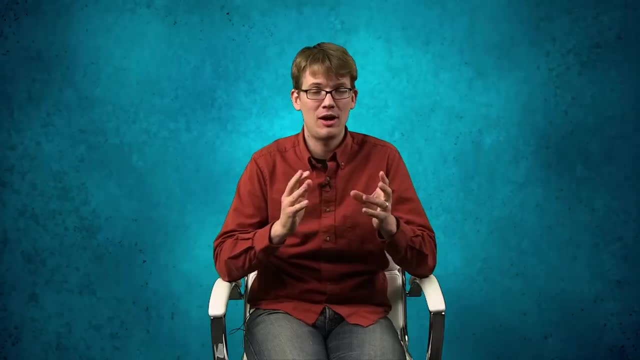 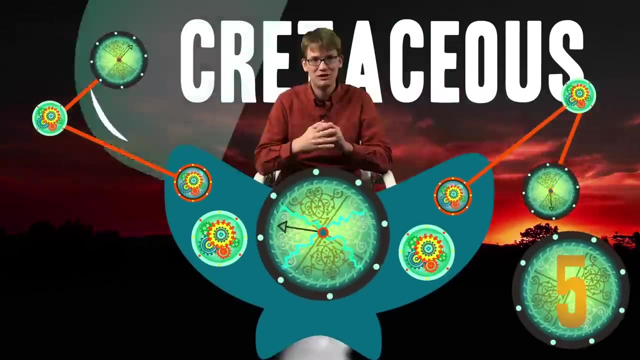 Off the coast of Mexico's Yucatan Peninsula, And you've heard of this one. It's where a giant asteroid or comet struck about 65 million years ago and that kicked off the Cretaceous-Tertiary extinction. You know this one. It's the one that killed off all the non-avian dinosaurs and ushered in the glorious age of mammals and birds. Mammals and birds- The K-T extinction, as it's also known- killed off half of all genera and 75% of species. 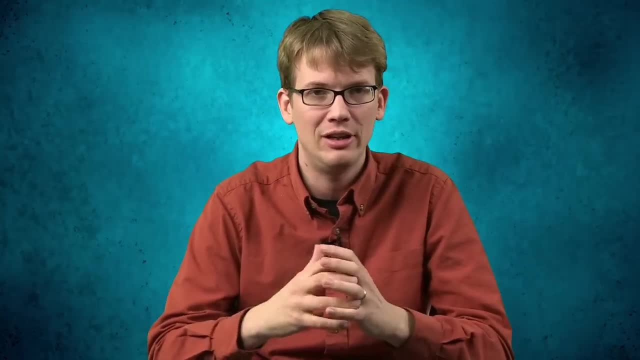 And while the giant asteroid impact winter-themed Earth, it also killed off half of all species. And while the giant asteroid impact winter-themed Earth, it also killed off half of all genera and 75% of species. Okay, now this nuclear theory is the leading one. 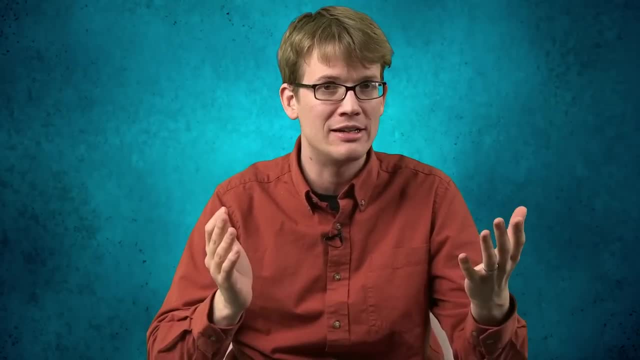 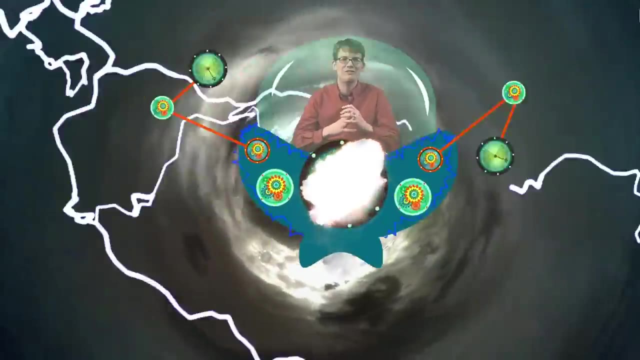 It's by no means the only one. Also happening at the same time, there was a giant volcanic eruption in India that may have caused massive global warming, And that final extinction brings us back around to today, where 99% of the species that have 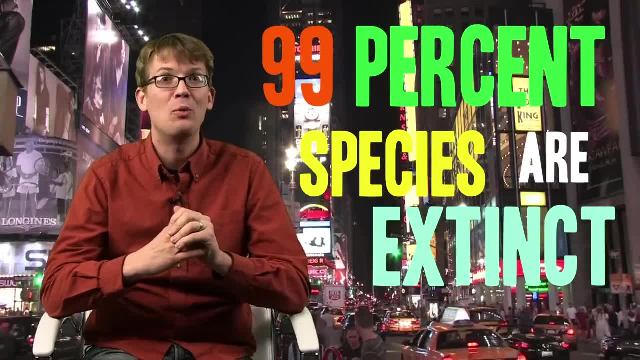 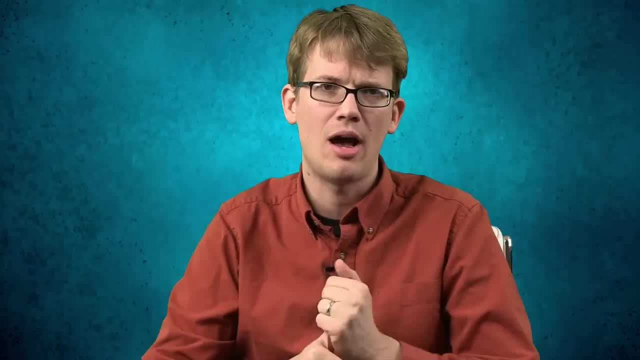 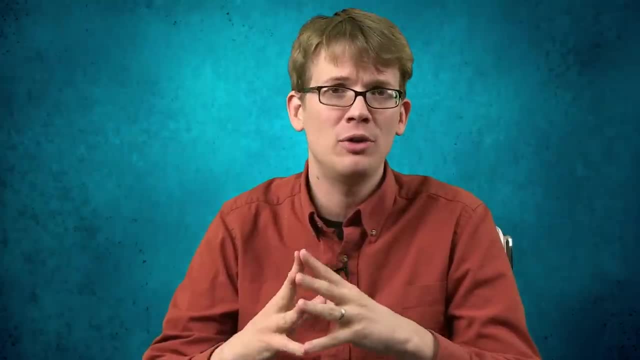 ever existed on this planet are extinct, But we aren't. WE ARE THE ONE PERCENT. Not. lucky for us, in the history of humanity we haven't had to deal with any giant comet strikes or supervolcanoes, but we do have to deal with a possibly equally destructive force. 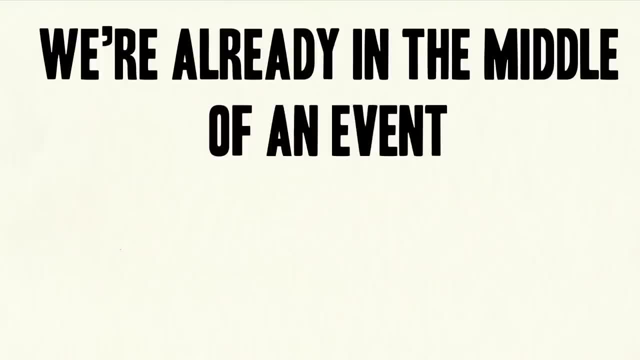 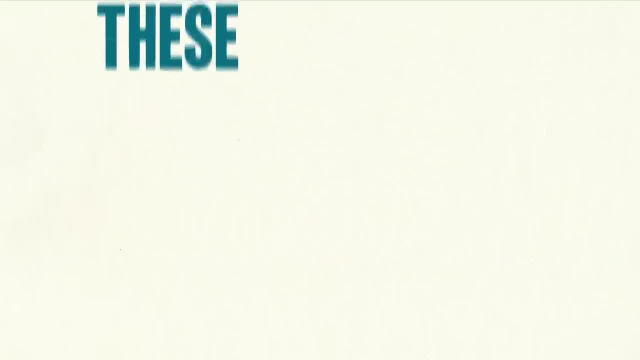 each other. Some scientists think that we are already in the middle of an event that's moving faster than the KT extinction. But instead of being driven by continents or volcanic eruptions, these extinctions are being caused by rising CO2 levels, habitat destruction, invasive species, pollution and 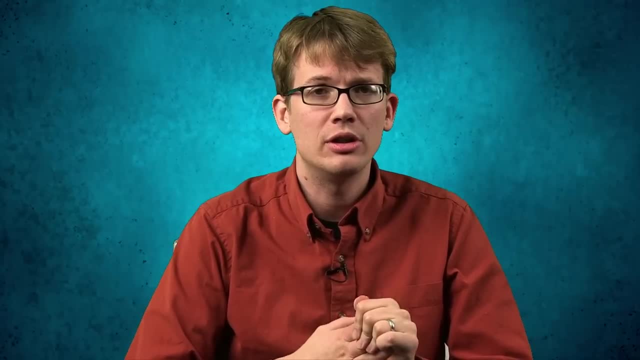 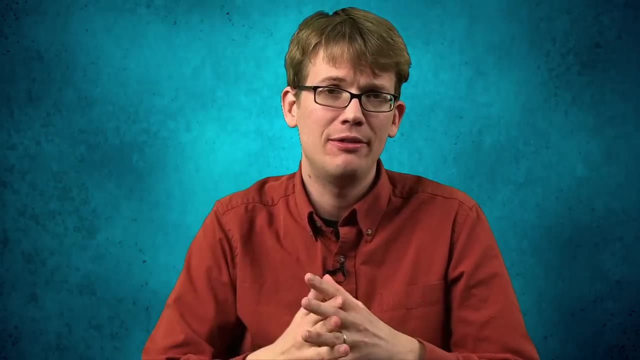 over-harvesting. We already know what changes in global temperature can do to a planet. Click over here for information on that in our climate change video. A normal extinction rate for our planet is about 10 to 25 species per year, and we're 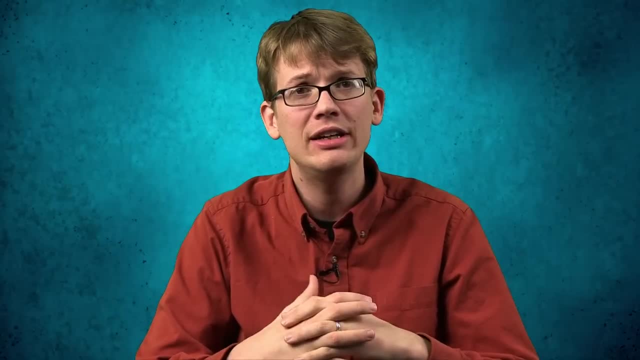 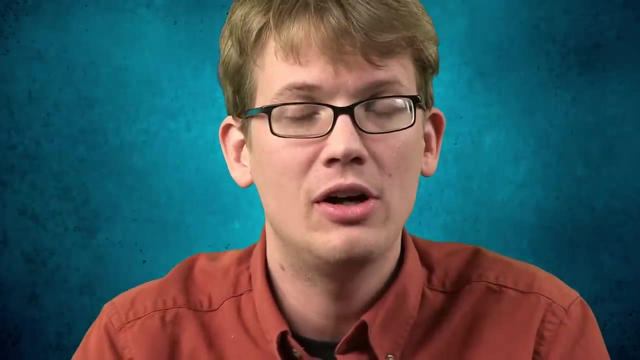 already doing about 100 times that. So clearly, 7 billion of us here on this planet are having a pretty big impact. I guess the question that remains for us to answer is: what are we going to call this sixth mass extinction event? 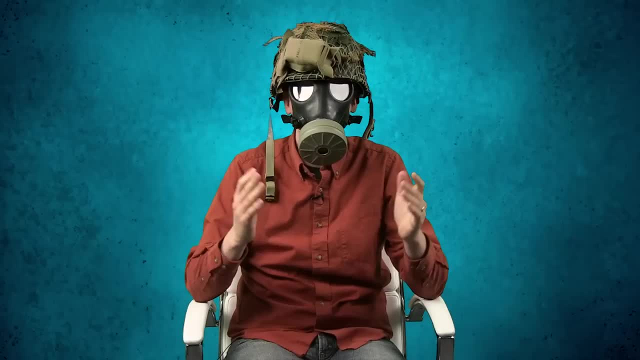 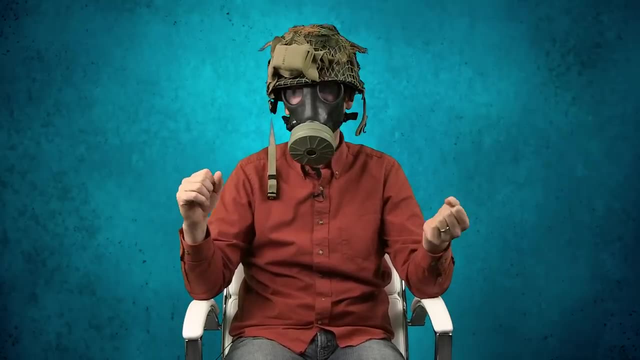 And I would love for you to leave ideas for that in the comments. Thank you for watching. Of course, there's sources for all of our information down in the description. because we are scientists here, we, We do. It's hard to breathe. 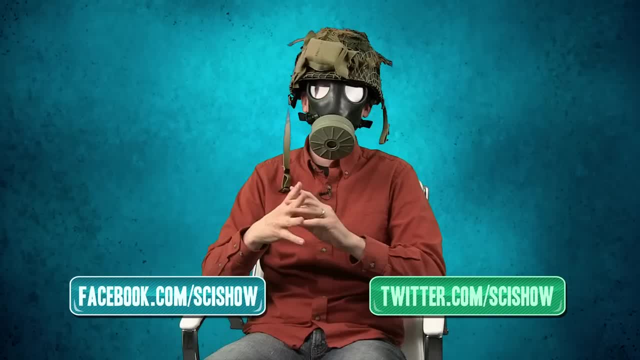 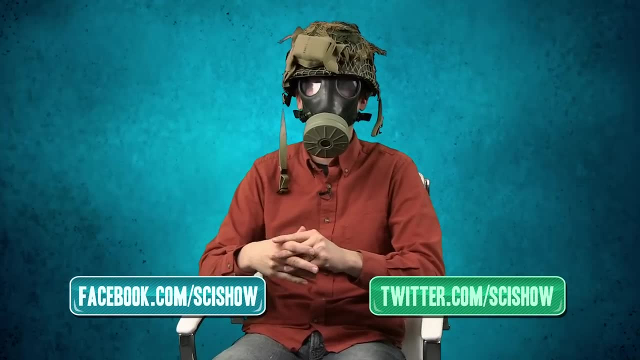 We are around if you have questions or suggestions on Facebook, Twitter and, of course, in the YouTube comments below. And if you want to continue to be smarter and know more about the world, go to youtubecom: slash scishow and subscribe. Goodbye. Bye, Bye.